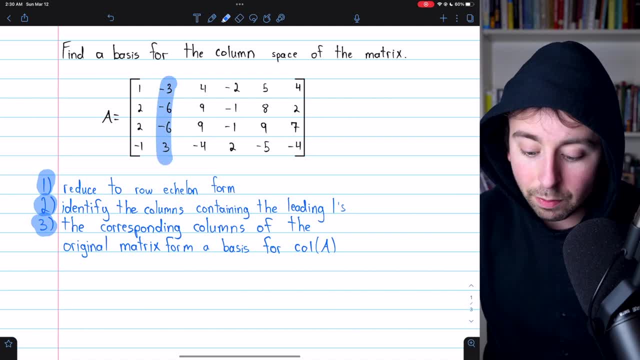 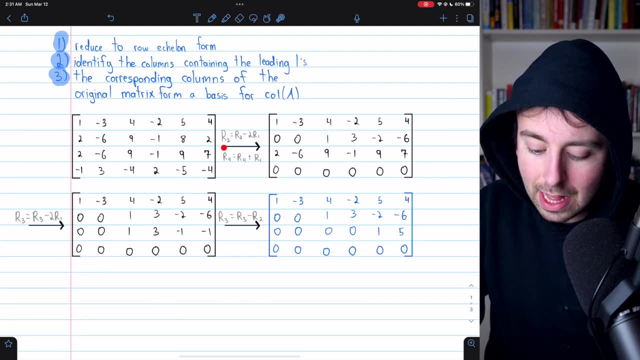 contain the leading ones, then it will be the second and fifth columns. Alright, here is our original matrix and the elementary row operations we performed to get it into row echelon form. I won't explain these all in detail. I assume you're comfortable with this process. I'll explain, say just, 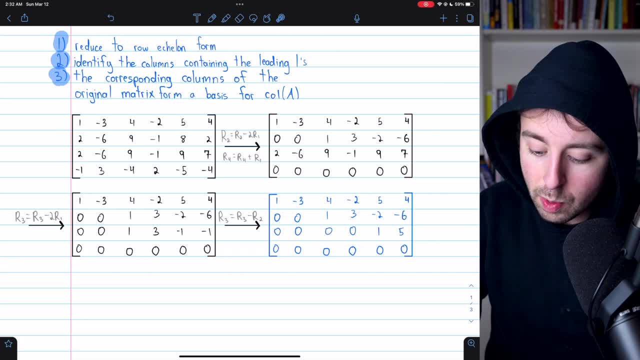 this step here to make sure my notation is clear. When we go from here to here, what we do is replace row 3 with the row 3, minus 2 copies of row 1.. So to go from here to row here to here, we're subtracting two copies of row 1 from row 3. And in the end we get this: 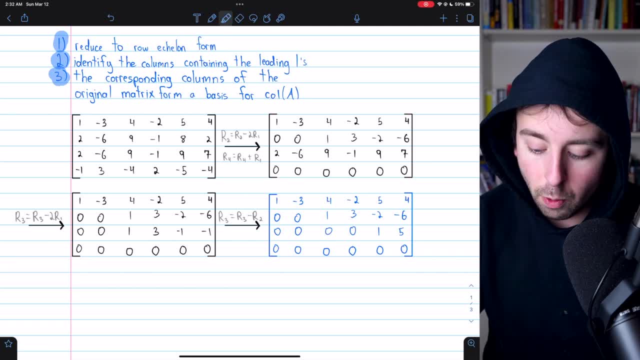 row echelon form. It's not reduced row echelon form. like this, leading 1 isn't in a column of all zeros, which would be necessary for it to be reduced row echelon form. but we don't need reduced row echelon form to find a basis for the column space, so we can stop there. So now that 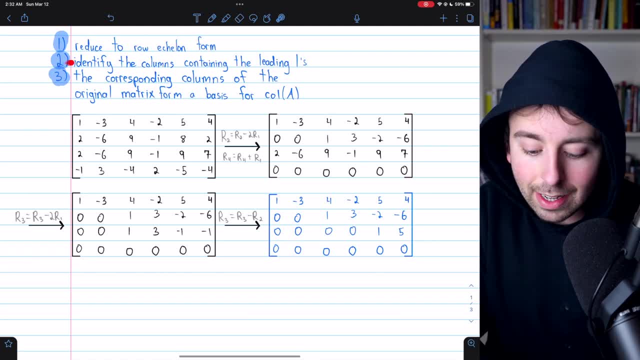 we've got it in row echelon form. the second step is to identify the columns that contain the leading 1s. The leading 1s are in the first column, in the third column and in the fifth column, right You. 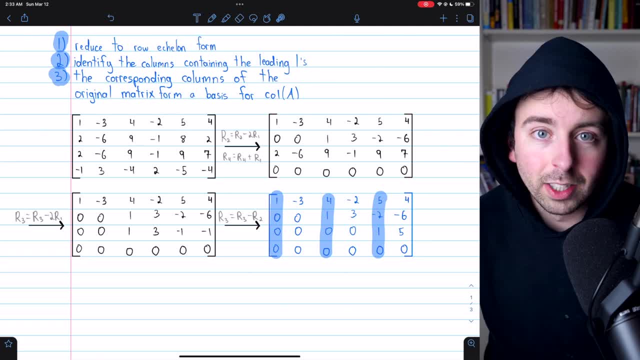 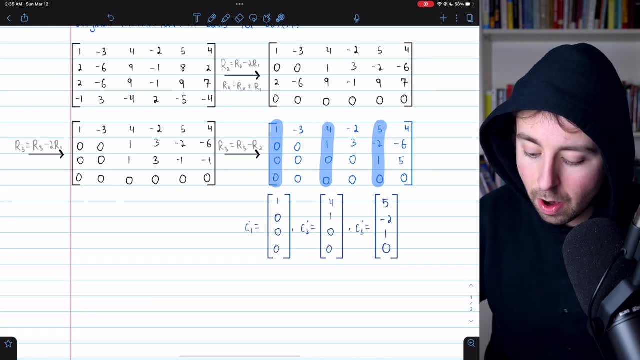 see all those leading 1s. so those are our columns of interest And we may choose to write those as such: c prime 1, c prime 3, and c prime 5, using primes here because these are column vectors from. 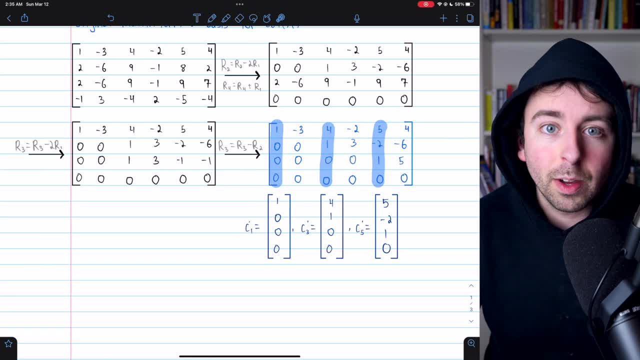 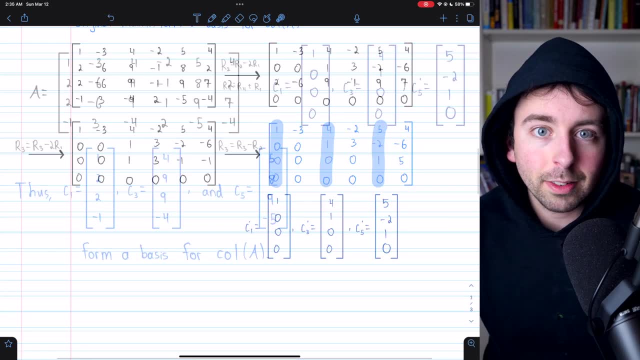 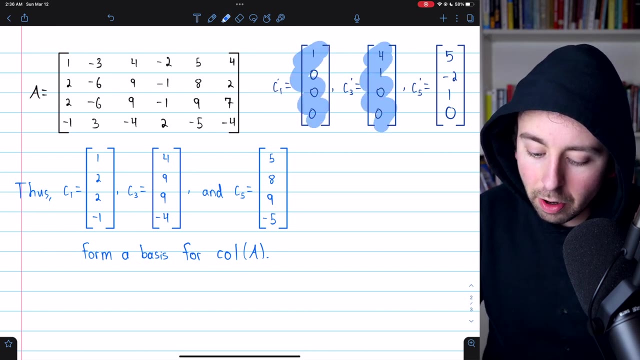 the echelon form matrix, not the original matrix A that we're interested in, But we now have sufficient information to find a basis for the column space of the original matrix. This is our original matrix A and, as we saw in the echelon form, it was the first, third and fifth columns that contained the leading 1s. Thus, 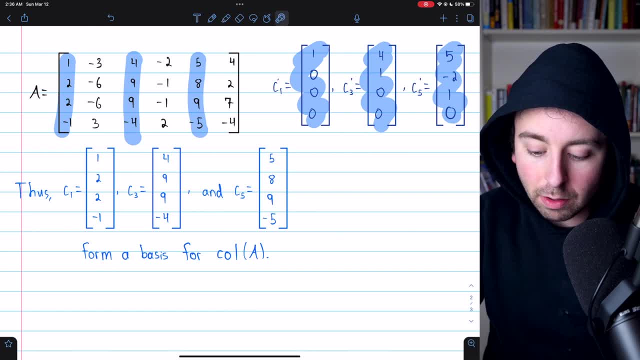 it's the first, third and fifth columns from our matrix A that will form a basis for the column space, And that's it. Once more, it's not the column vectors from the echelon form that make up a basis for the column space, but it's the